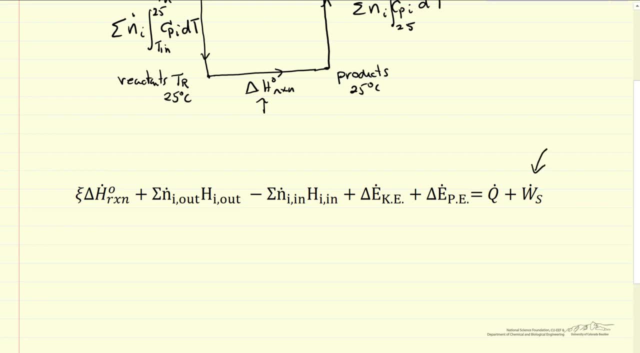 Next we need to doFE, So we've moved it through other terms. This is: and the dot means per time, This is work per time, so kJ per second, and this is shaft work, And this term is the heat added, again per time, So heat added per second, shaft work per second For most. 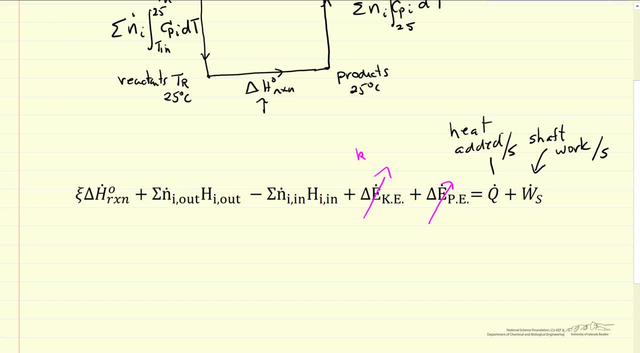 chemical reactors. the change in positron xerma is change in kinetic energy, so this is kinetic energy and this is potential energy. Those terms aren't going to be important, and so for this case we're going to look at them as zero. So for the left side, the extent. 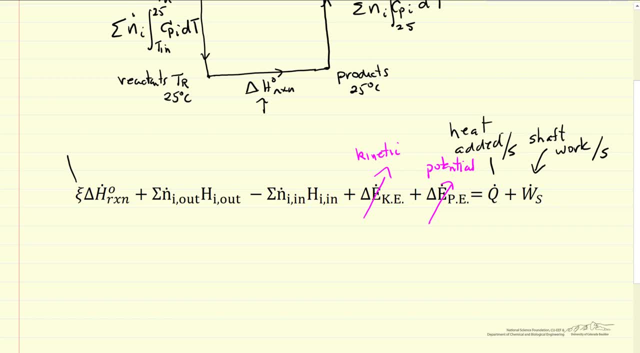 of reaction and there's multiple ways that this is defined in the literature, so I'm just going to show one way. So we have some reactant gonna rate the flow rate out, flow rate in, divided by its stoichiometric coefficient. 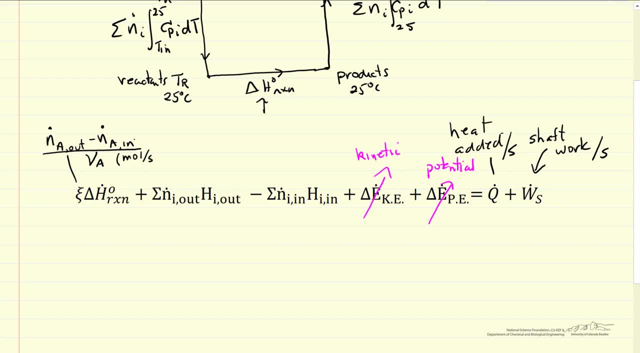 where, in this case, we're gonna have the stoichiometric coefficient of units of moles per second, so that the extent of reaction is dimensionless. Other textbooks will define this extent of reaction having units of moles or moles per second. 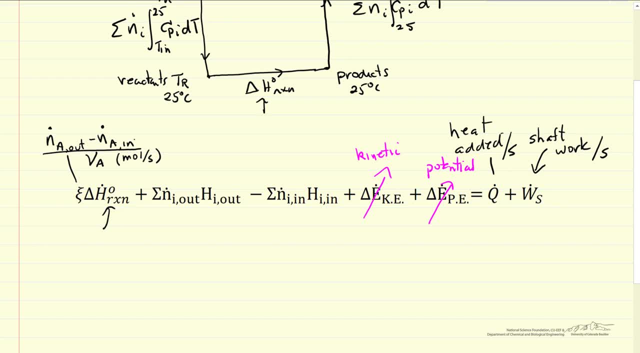 The heat of reaction term is the standard way that we calculate this sum of stoichiometric coefficients times heats of formation, standard conditions, each component, and then again to make it per time. So this is the values we look up from tables at 25 degrees C. 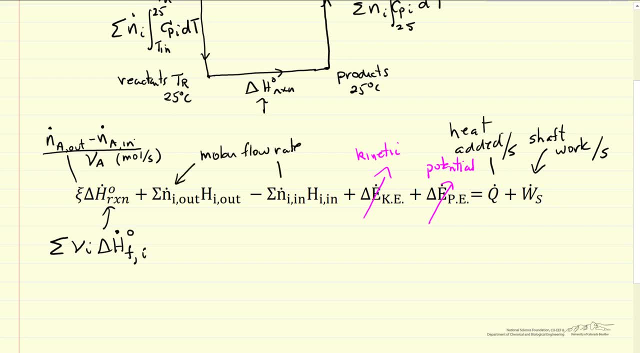 So, to make clear, this is a molar flow rate, as is this term here, one flow rate in the other flow rate out for various species And this term is enthalpy for mole for each species. In this case it's integral from our reference temperature. 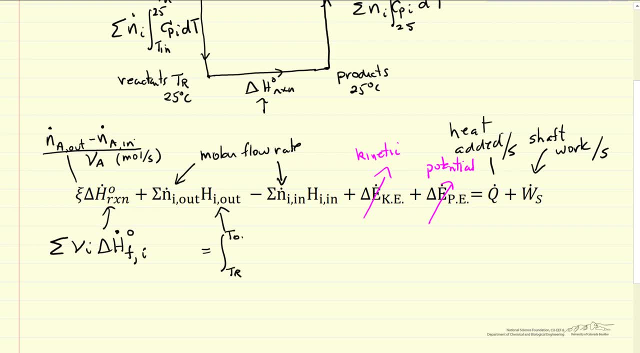 here we're using 25 degrees C to the outlet temperature. heat capacity of each component, DT, where the heat capacity typical form would be a constant. a second constant times temperature. a third constant temperature squared. a fourth constant temperature cubed. 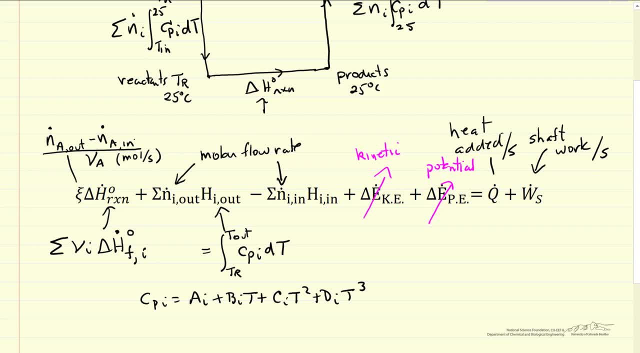 but there are other forms that are also used for heat capacity And likewise the enthalpy. the temperature squared, the heat capacity squared, the enthalpy coming in is in this case evaluated from reference temperature to inlet temperature. heat capacity DT.